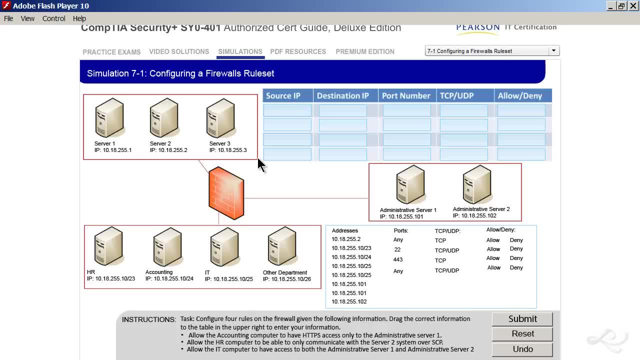 It depends if you're working in an operating system or a SOHO router with built-in firewall or a more advanced firewall appliance. So this is more of an abstract simulation of what you'd be doing with the firewall rules, As long as you know the basic information. 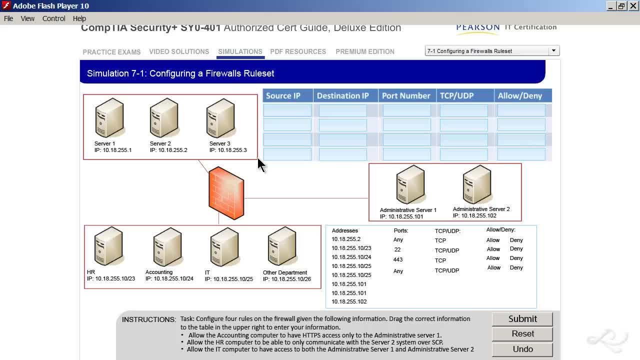 for the firewall rules, then it's just a matter of semantics and getting the syntax correct or going to the right place and clicking the right dropdown menus. So you need to know how this firewall rule works. So we have this table of information here. 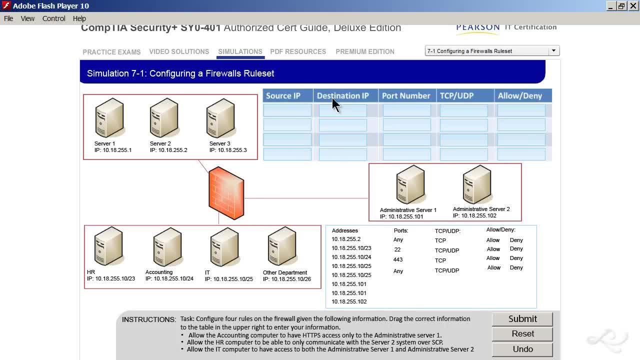 It's blank right now. We're going to fill it in. We have the source, IP destination, IP port number, whether it uses TCP or UDP mechanisms or both, and whether you're allowing or denying that access, And we fill this table based on the instructions that were given down here. 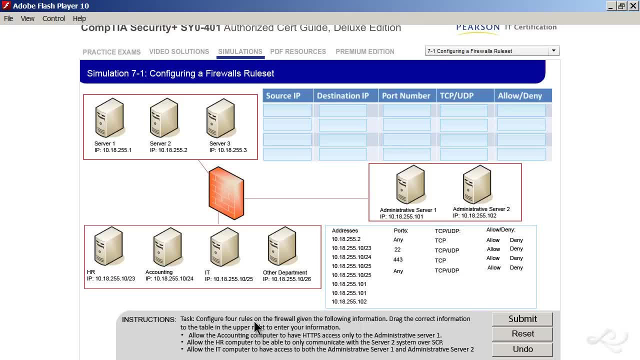 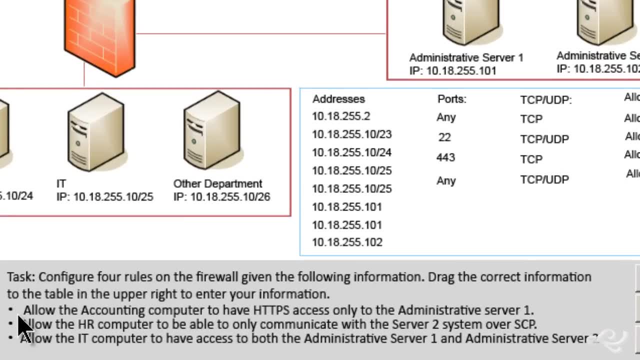 The task. configure four rules on the firewall, given the following information. The first rule is allow the accounting computer to have HTTPS access only to the administrative server one. So let's say that your boss tells you, okay, the accounting computer needs to. 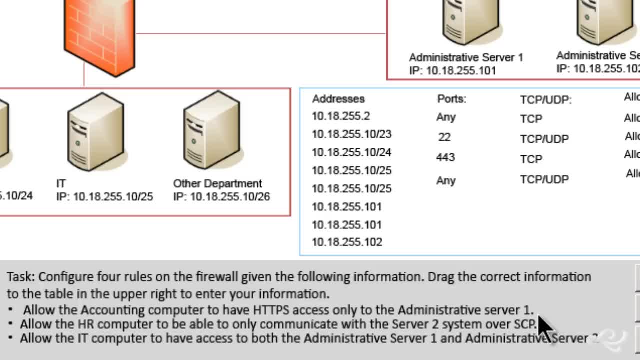 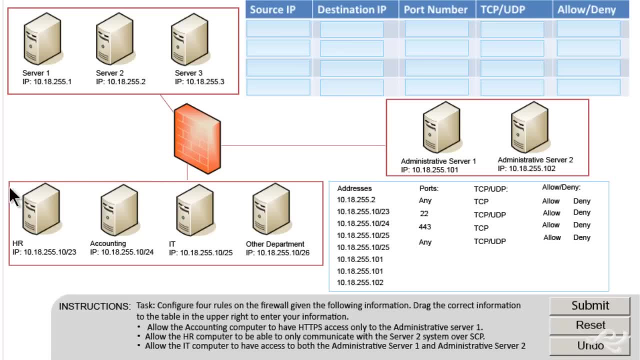 connect to the administrative server, but we only want it to have access through HTTPS. Well, who are the players? Here's the accounting computer, That's on one leg of the firewall, in the general area of the LAN, And here's the administrative server, on another leg of the firewall. So, to get through the 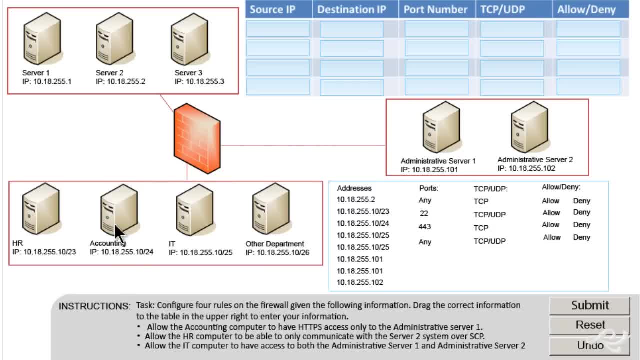 firewall. you have to create that firewall rule for the accounting computer. So here's the IP address of the accounting computer and that's right here. We'll drag and drop that to the source IP on the first row of the table. The destination IP is the. 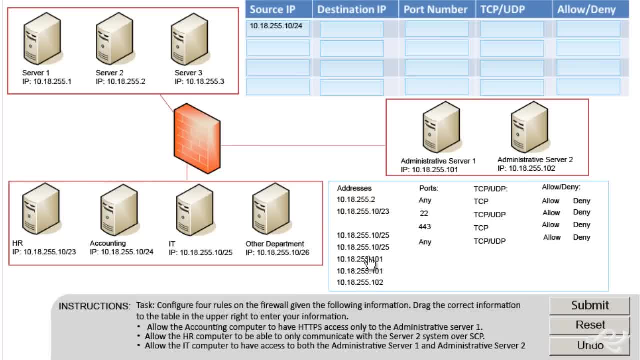 administrative server: .101.. So we'll grab that IP, drag that into the destination box. Now, port number: what are we going to use? Well, it tells us we want to use HTTPS And the port number for that is 443.. So we'll grab that and drag it in. 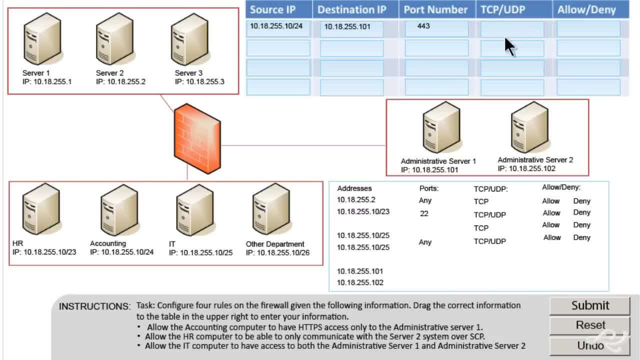 Now are we using TCP or UDP as the transport mechanism? Well, HTTPS, like HTTP, uses TCP and TCP only, And we want to allow, so we'll drag that over there. We're allowing the accounting computer access to the administrative server on port 443 with a TCP connection, No other. 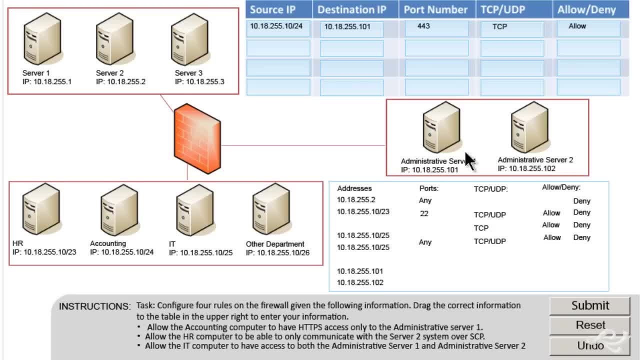 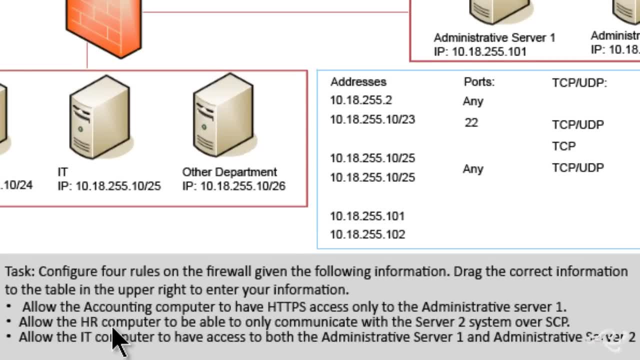 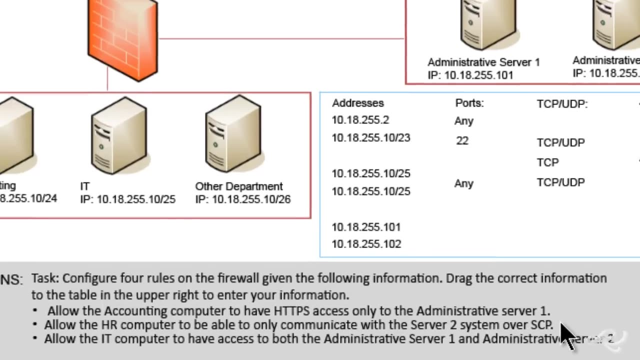 connections are going to be allowed between the accounting computer and the administrative server. The firewall will block those. So the first rule is done. Second rule: allow the HR computer to be able to only communicate with the server two system over SCP, Worded a little bit differently. 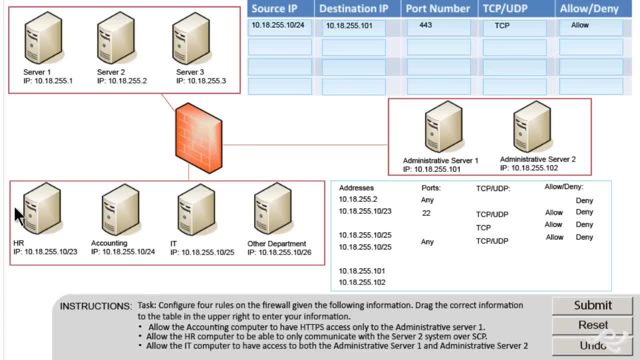 but same type of idea. We have two players, the HR computer and server two up here on the third branch of the firewall, And we want to use SCP as our protocol. So we're going to grab this IP address. That's the source IP. This guy's going to be the destination IP And now we need the. 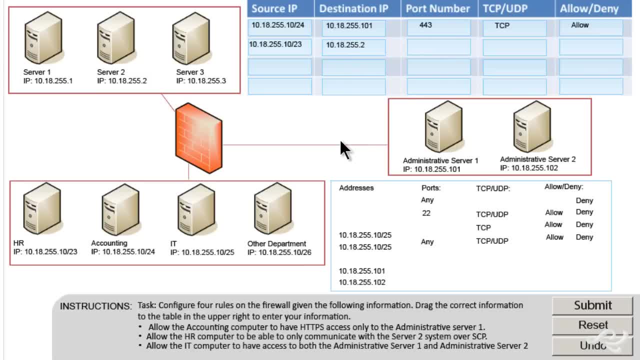 port number. Well, what does SCP use? It's based off of SSH Secure shell, port 22 only And that also is TCP only as the transport mechanism And we select allow And that firewall rule is done. Again, keep in mind that the syntax you might use if 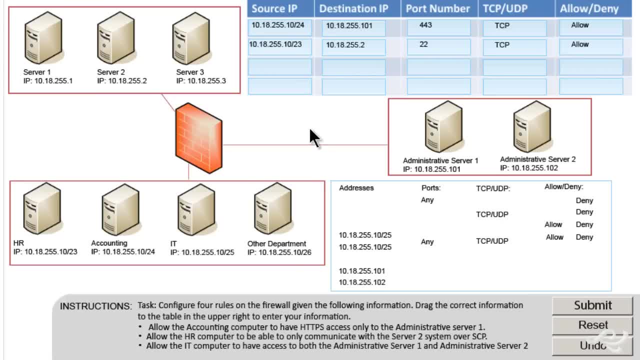 you're in the command line will be different. You know you can use net SH in windows or you could use the windows firewall with advanced security, or you might have a firewall built into your Soho router. Getting into bigger networks, you might have a. 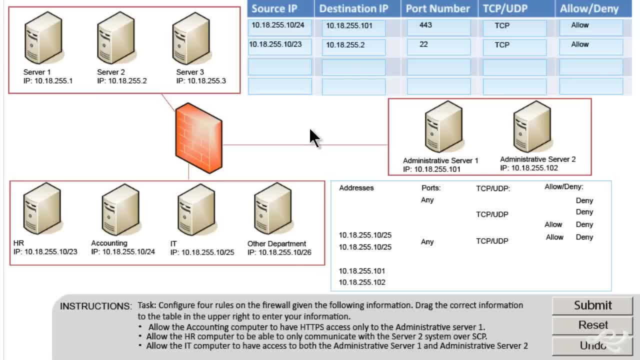 different type of firewall altogether, something from Checkpoint or from Juniper networks or Cisco or what have you. The graphic user interface or the command line syntax will be different depending on the firewall you're working with, But the general rule here will remain the same, You'll. 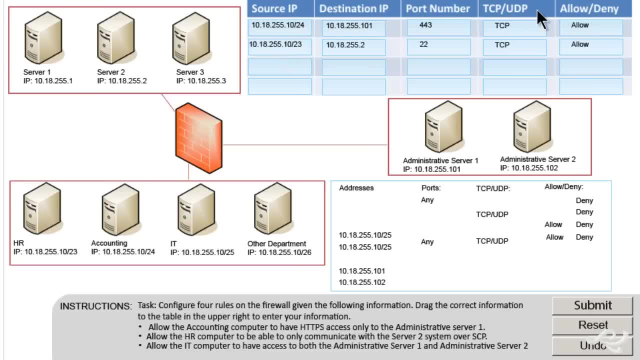 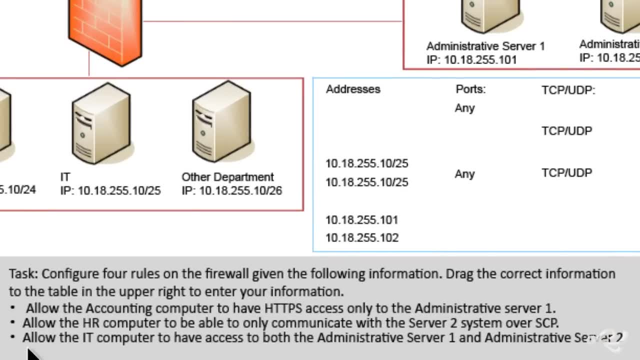 have a source, IP destination, IP port number, a transport mechanism and whether that is allowed or denied. So let's go to the last two rules, which are basically the same as the first two rules. So let's go to the last two rules, which are basically the same as the first two rules. 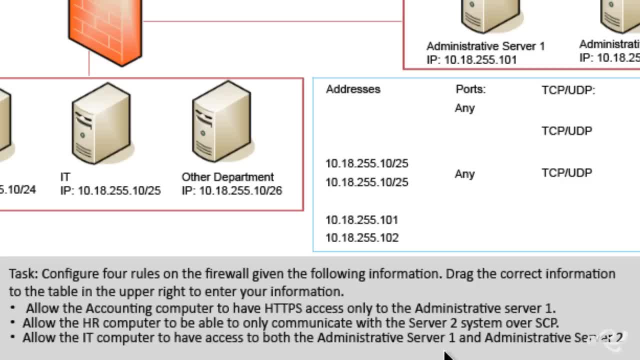 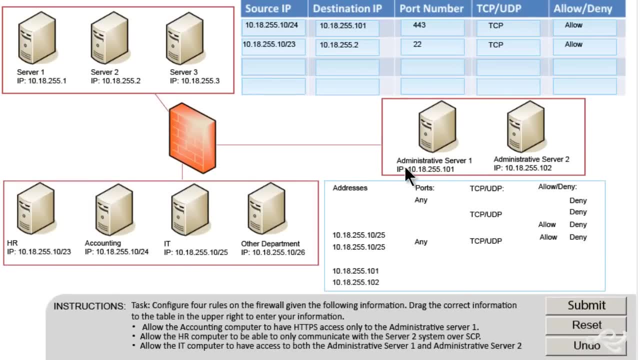 So let's go to the last two rules. Allow the IT computer to have access to both the administrative server one and administrative server two. Here's the IT computer And here's administrative server one and administrative server two. So that's who we're going to connect to. Here's the IT IP address. We'll grab that. Go to source IP. 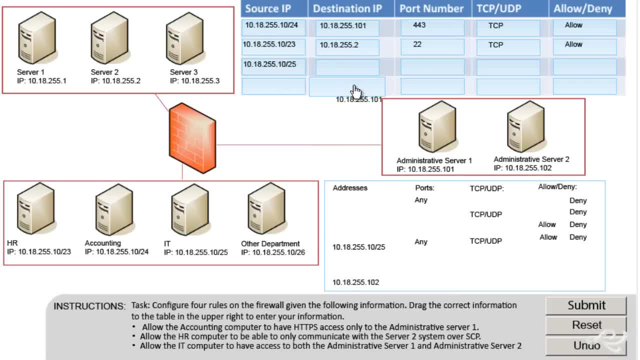 Then the destination is this guy .101.. Ports any Why? Because it just says the IT computer should have access to both of the servers. It doesn't say only with a specific protocol, And IT people are generally allowed access to servers through any. 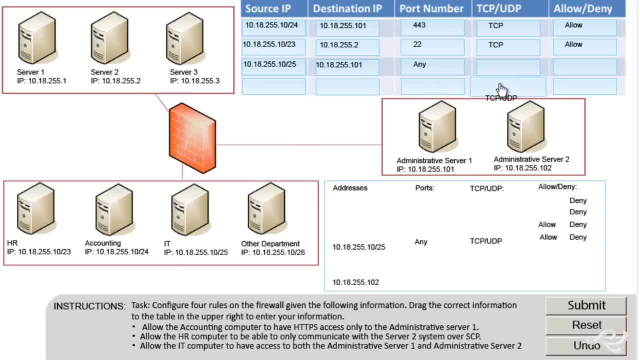 port. So we say any and we do TCP and UDP. So either transport mechanism and allow, And the second half of that is again going to be the same IT computer And then the administrative server two, which is one, 102.. Any for port number, TCP and UDP and allow. 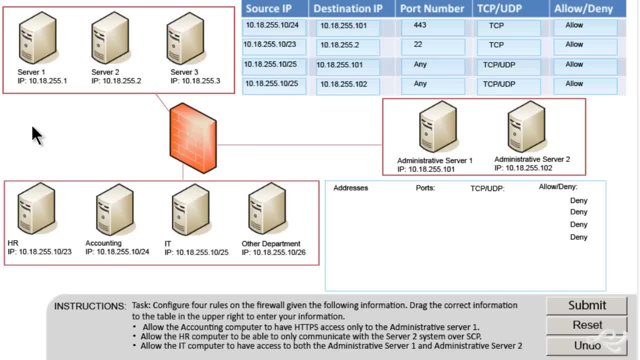 This is just an example. This is just a simulation, But you could be called upon to make different connections between different computers with different ports. For example, let's say the HR are only allowed access to server two With TFTP. Well, instead of port 22,, that would be port 69.. TFTP is the trivial file transfer. 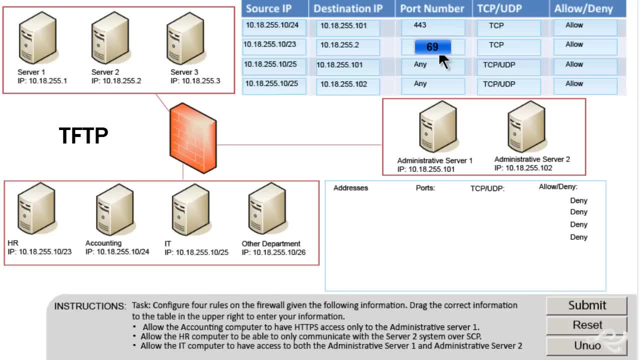 protocol. It could be they're just sending very basic information over TFTP. It could be for grabbing an image when booting off the network or something like that, And it's something that the user doesn't even do. It could be just the computers doing it, And so TFTP would use port 69,. 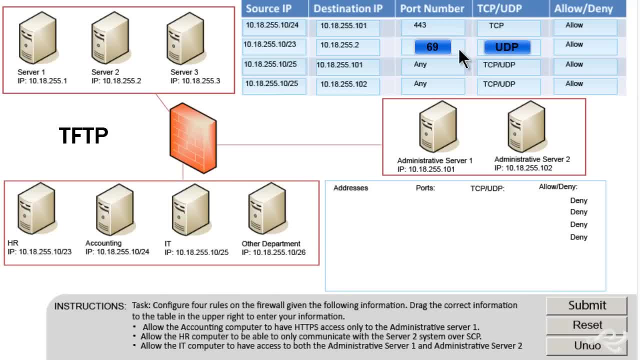 and that would actually be the same thing for the IT computer. So that's the trivial file transfer protocol. But then you would have to have a UDP transport mechanism as opposed to TCP. So it could be anything You might connect with a syslog server. Then you would want it to be port 514 and most likely UDP.